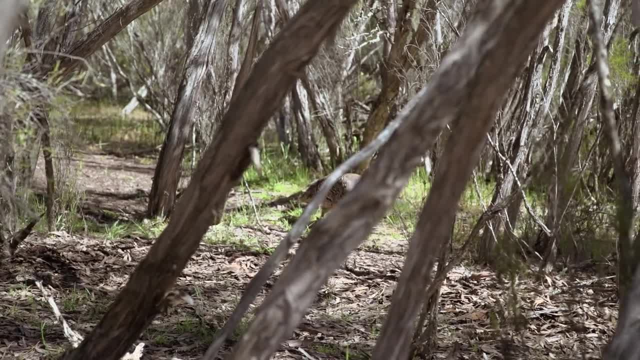 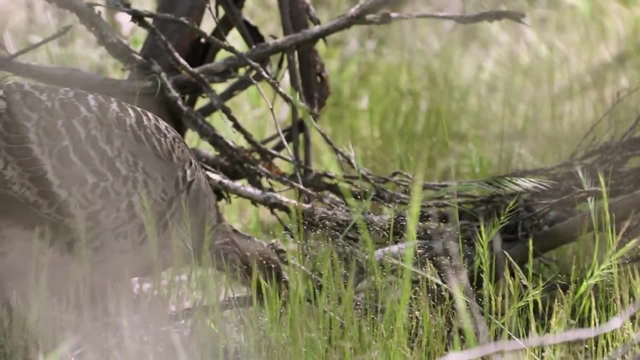 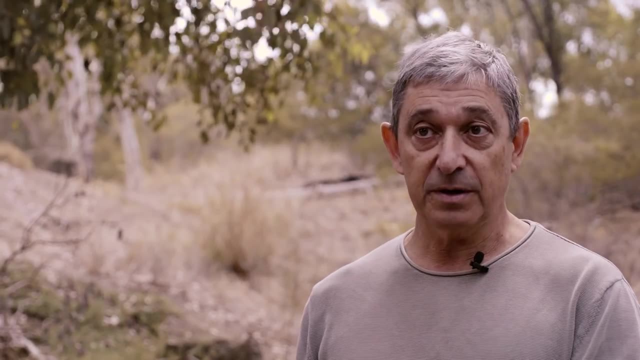 heat. All the others use body heat. The Malifow belongs to an extraordinary family and it is the most extraordinary member of that family. Birds such as the Australian Brust Turkey scrape together a whole lot of leaf litter and let it slowly rot because they're in very 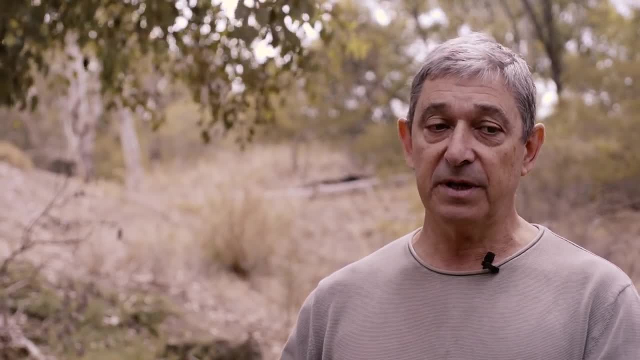 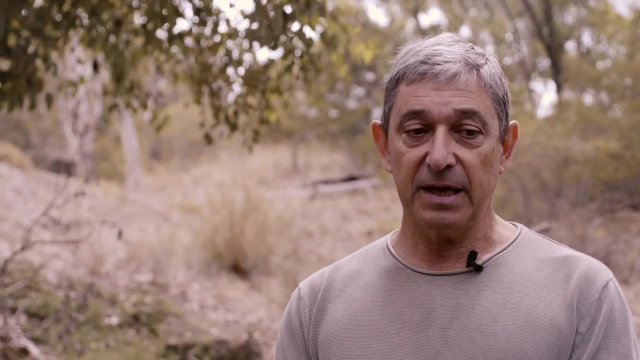 very moist environments and if they scrape together a whole lot of leaf litter it rots. and then they go and they have a look and they find a warm spot. The Malifow has taken it another step, or actually another couple of steps. It also rakes up leaf litter, but 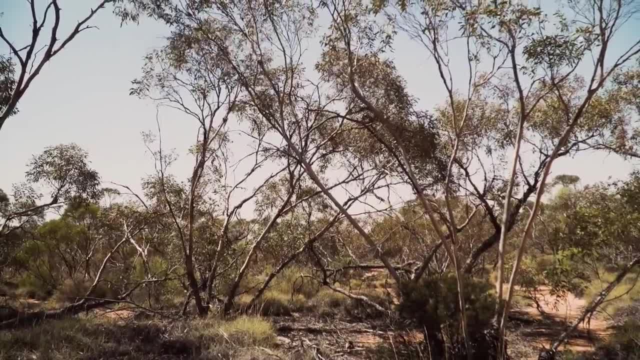 what makes it unusual is that it's the only Megapode to live in an arid environment and just scraping up a whole lot of leaf litter. it rakes up a whole lot of leaf litter. It's the only Megapode to live in an arid environment and just scraping up a whole lot of leaf litter. 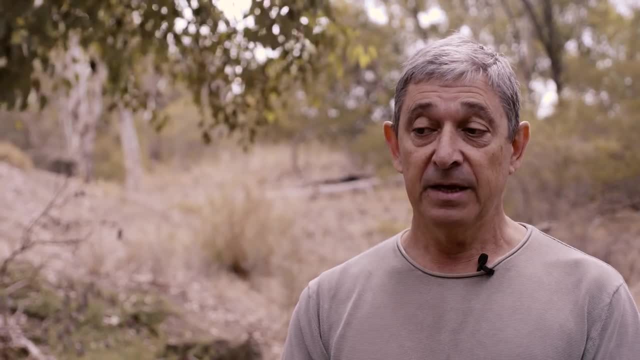 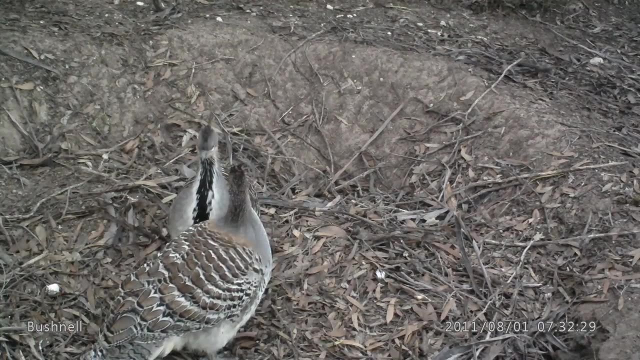 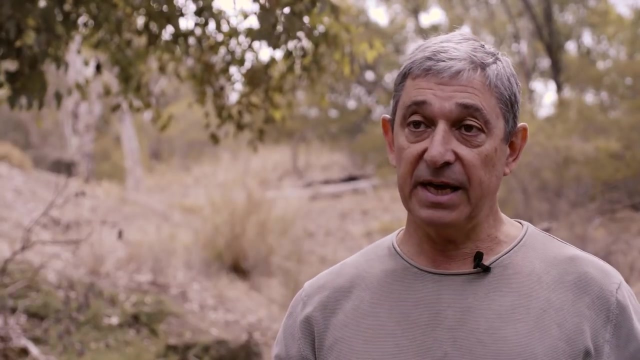 wouldn't do very much at all, because it would just dry out. So what the Malifow does is it first excavates a hole, fills it with leaf litter and then waits until that leaf litter is completely drenched with water. Then it locks in all that water with a layer of sand. 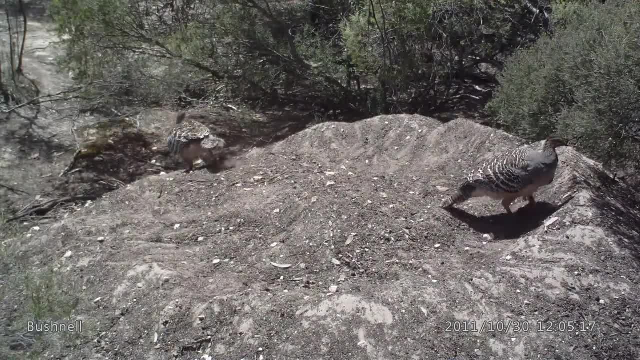 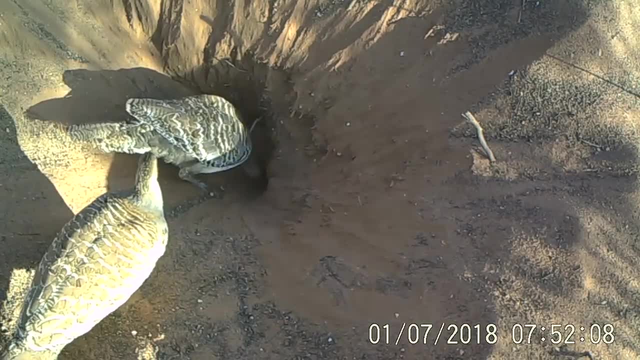 over the top And that prevents the leaf litter from drying out and it starts to decompose and generate heat, And then the birds dig down and lay there. And then the birds dig down and lay there. And then the birds dig down and lay there. 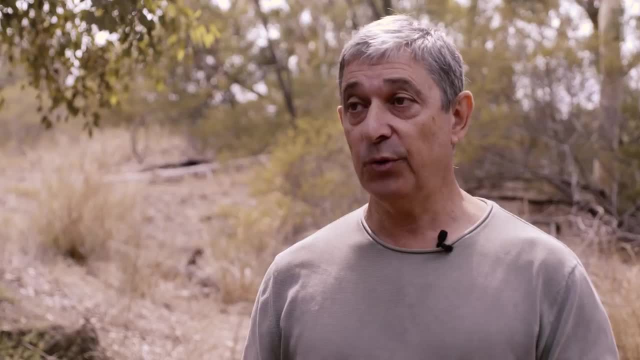 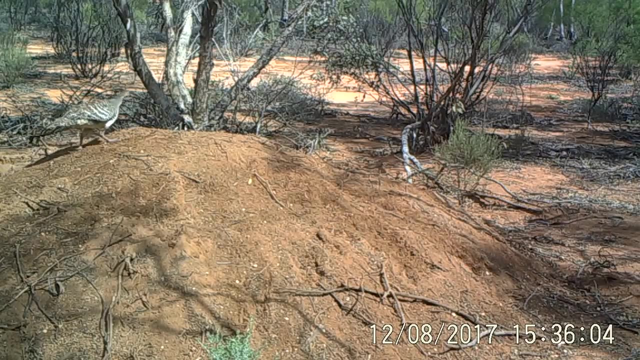 And that they're always in that warm sand. In autumn, a pair of Malifow will typically be walking around and every now and then the male sees a bit of a hole or perhaps a mound previously used mound of Malifow. 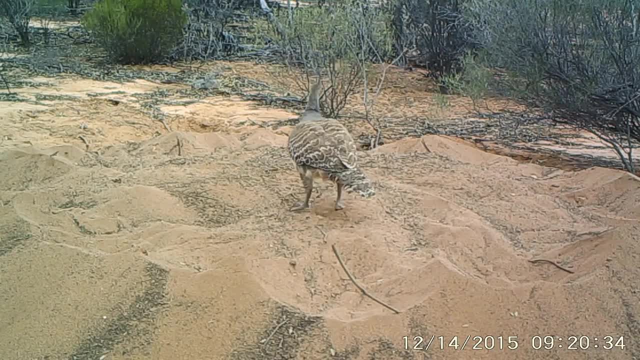 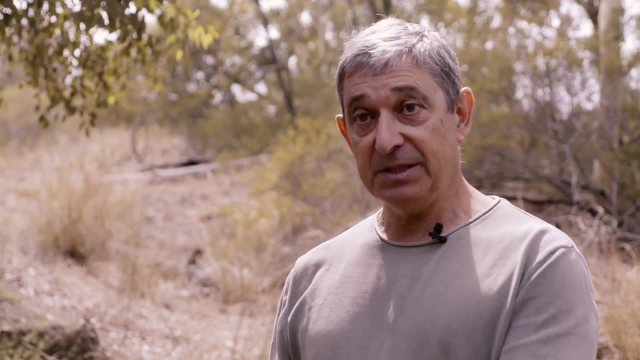 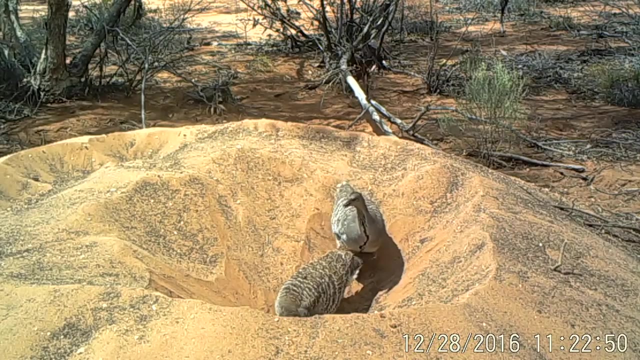 And they'll go up there and do a display and the female will come over and have a look and more often than not just keep walking. But when she finds the right mound, then they'll start work and they'll dig it out so that it's this big cone into the earth. 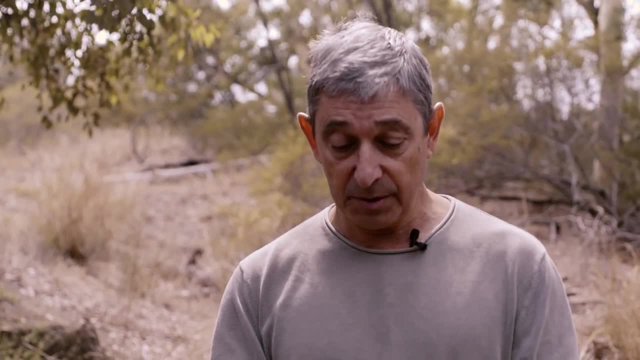 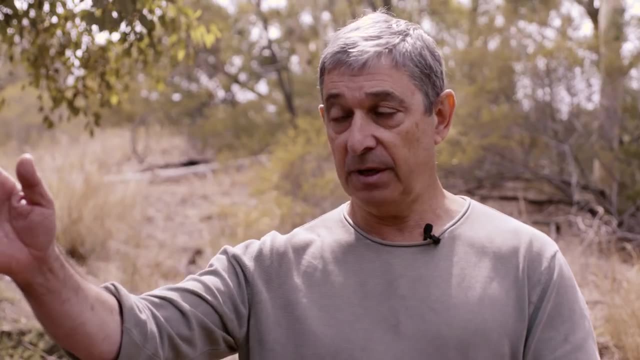 It could be up to a metre deep, this big cone into the earth with a square box down the bottom. and then the birds start to rake all the leaf litter and they work in a line so they won't necessarily just take the closest leaf litter. 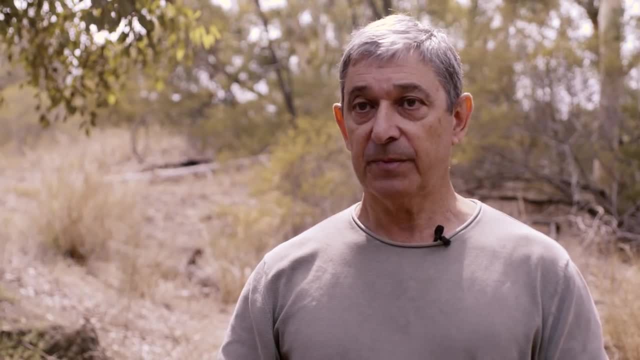 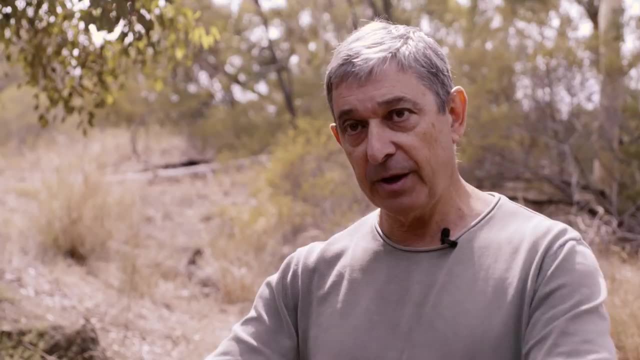 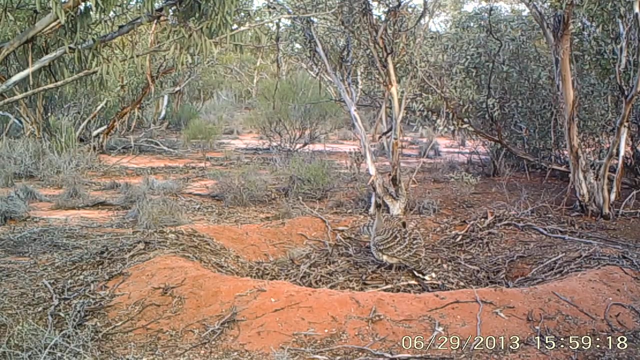 What they're actually doing is they're going to form a windrow and they're going to walk back and forward on this line of leaf litter until the whole thing slowly edges its way into the mound. So this can take weeks and weeks. They just rake it all in until they may have up to a cubic metre of leaf litter. and they're waiting for a big rain, One last big rain, to absolutely saturate all that leaf litter. When it occurs, they will quickly cover the whole thing in and lock in all of that moisture. And that's where the magic really starts, Because the moisture is locked in although it's bone dry outside and it starts to rot. 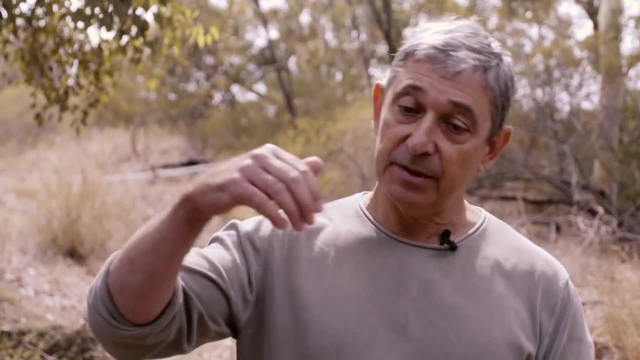 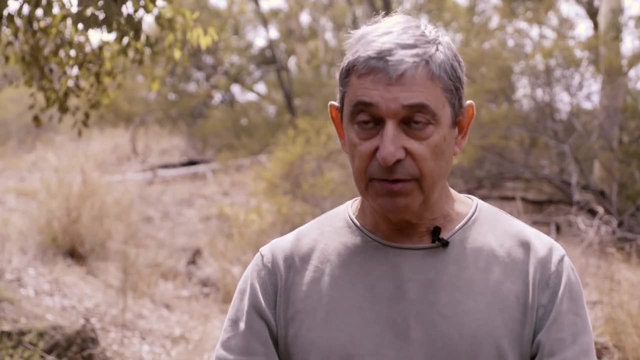 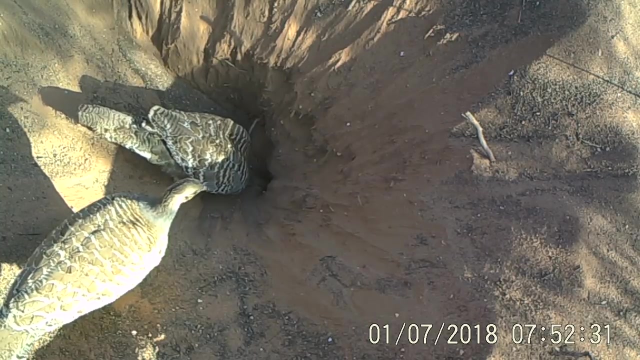 And as it rots it produces heat and the birds start digging down checking the temperature and as they do this, they're forming this plug of loose sand going into the leaf litter and we call that the nest chamber. So this plug of loose sand, dry loose sand, surrounded by rotting leaf litter. 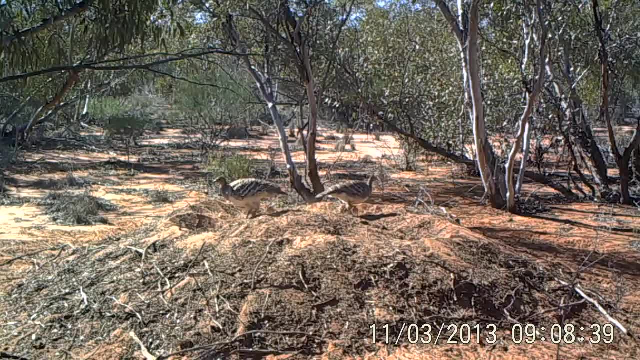 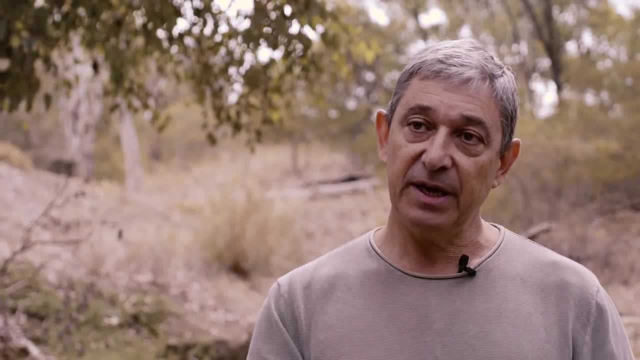 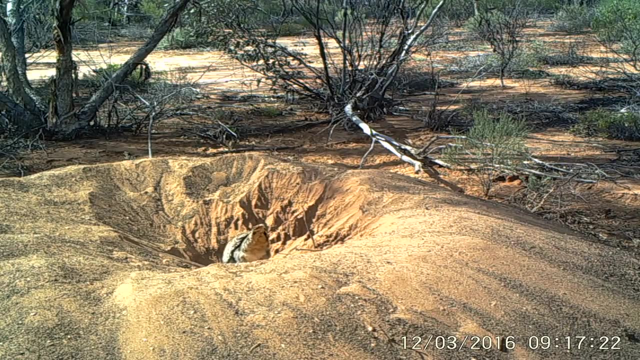 So they're surrounded by warmth. If you look closely at a- particularly the male, but also the female- going into the mound, what they do is they shove their head in and they take a bill full of sand. So presumably they have temperature sensitive membranes in their bill to measure the temperature of the sand. 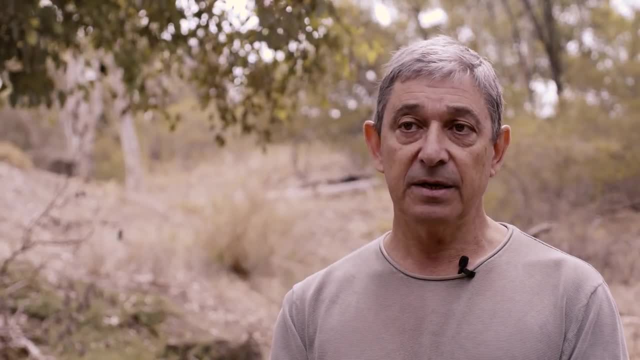 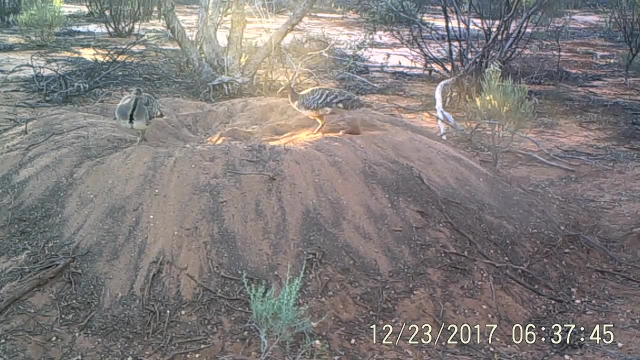 They might move a tonne of soil a day just opening and closing this mound. So when they're down there, they'll, they'll check the temperature and if it's too hot, then in the early morning they they open up the mound and let the heat escape to the atmosphere. 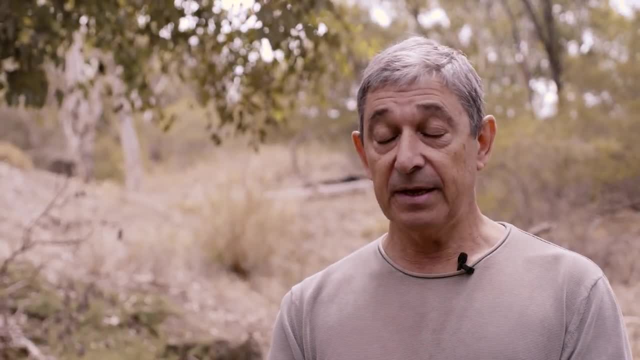 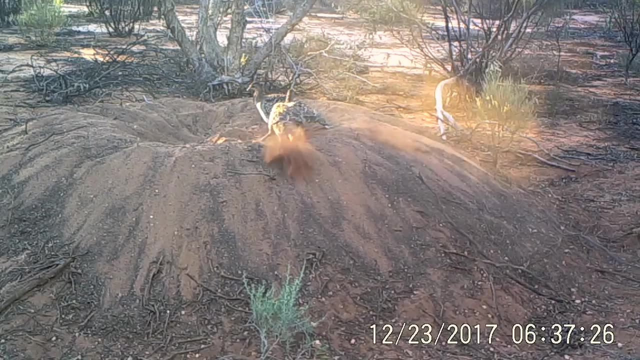 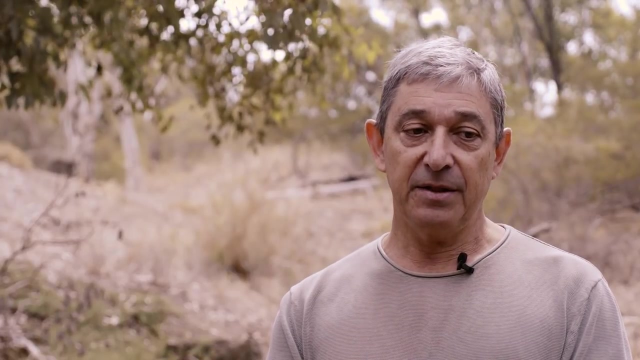 So even in, even in summer, it can get very fiercely hot in the Mallee, but the morning is pretty cool, So by opening up they can release a lot of that heat and cool the whole mass down. Later on the, the challenge is to warm the mound, and then they use an entirely different strategy. 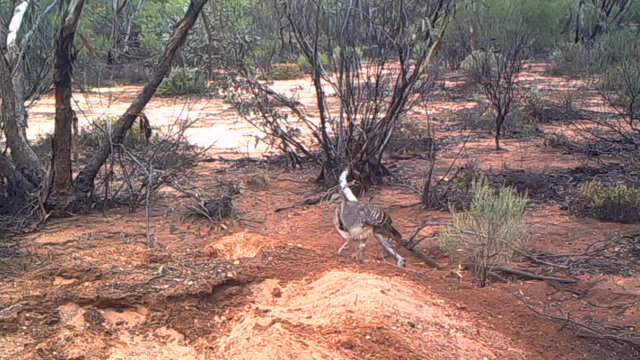 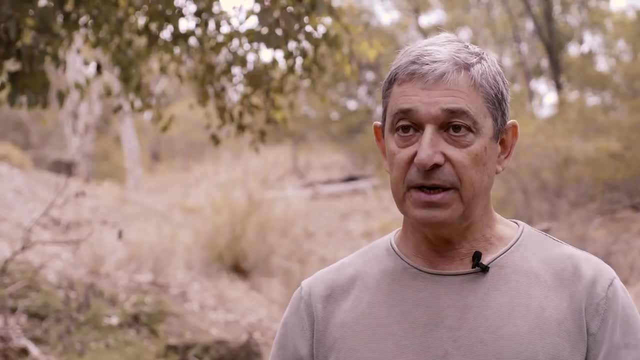 Later on in the season they open it later on, Later in the morning, and they lay all the sand out And then, as the sand, the surface of the sand, heats in the sun, they scrape that into the centre and then leave it for a while, let the surface heat up again and then scrape it, you know, back in. 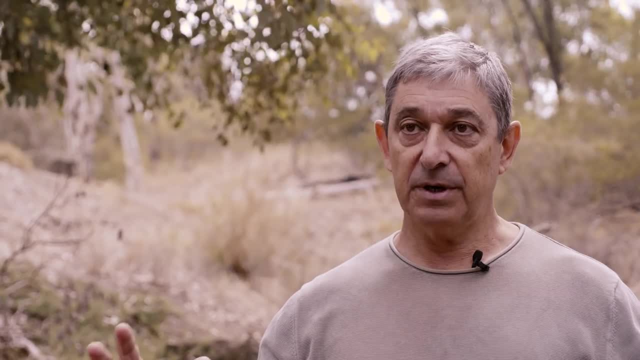 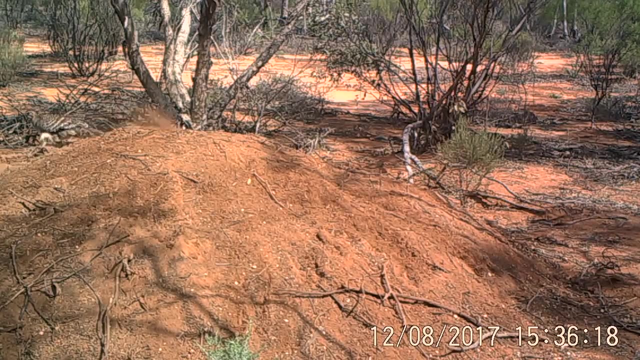 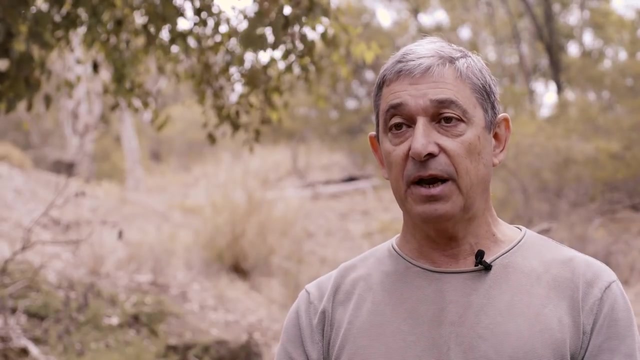 And in that way they have this big mass of warm- you know quite warm- sand above the eggs. that then heats the eggs to the required temperature. In terms of the working mound, they'd be about five metres across and at its height when the birds are really, you know, mounding it up before a rain or something like that. 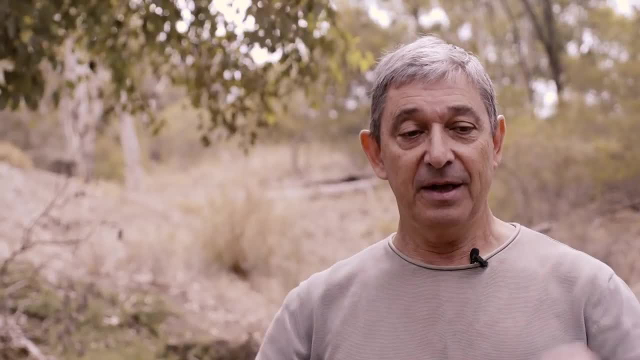 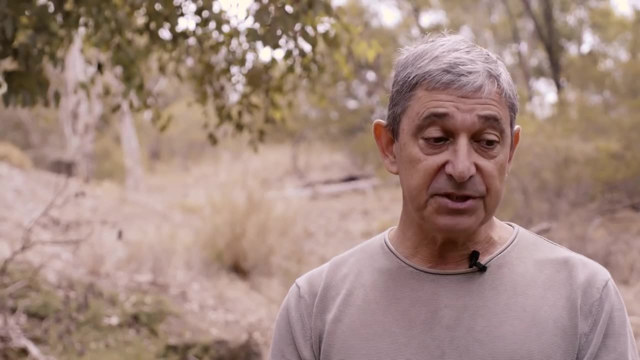 which can kill all the eggs, so that they're very steep and they'll put a lot of sticks on the top as well. they can easily be a metre high. So quite enormous structures really. These structures, once they're built, are really quite persistent in the landscape. 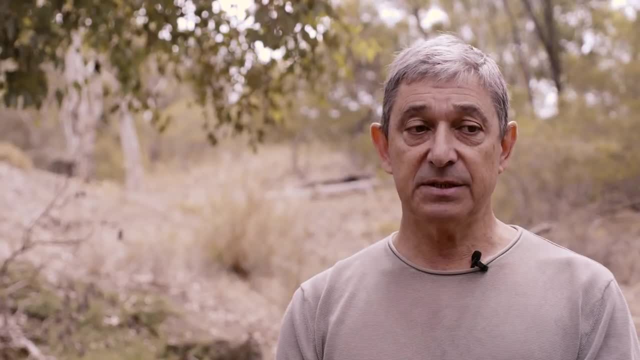 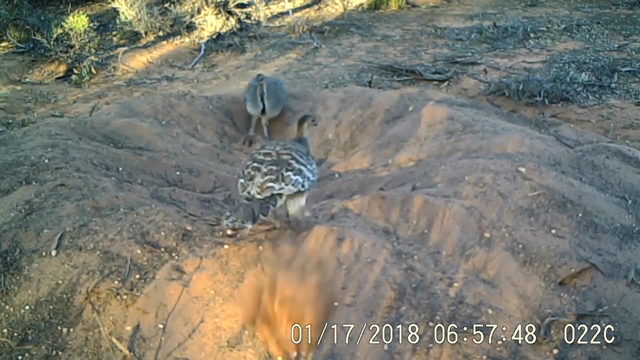 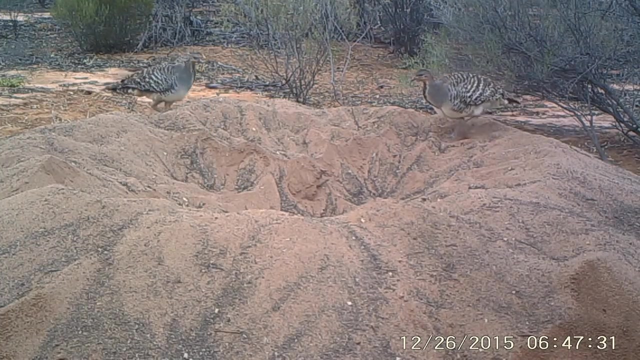 So what Malleefowl tend to do is to go to previous structures that have been used and renovate them. That's not to say they don't also build new mounds, And some birds just like building new mounds, But typically they reuse older mounds. 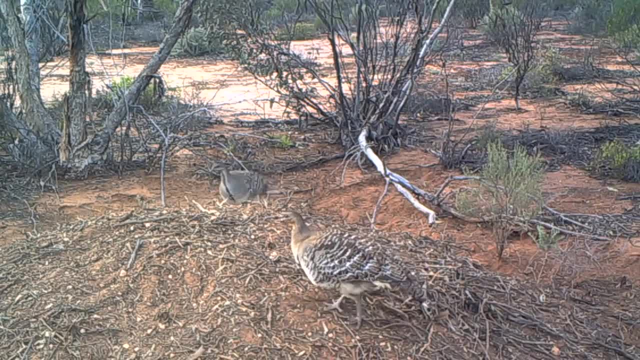 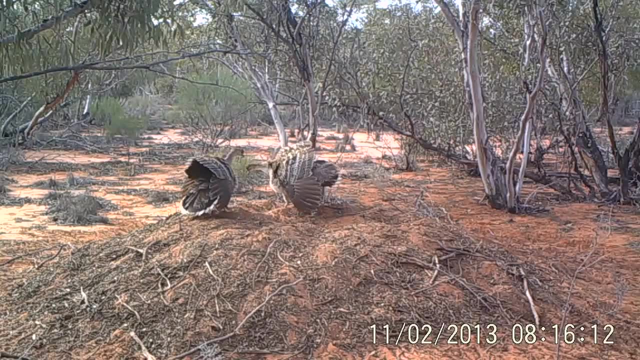 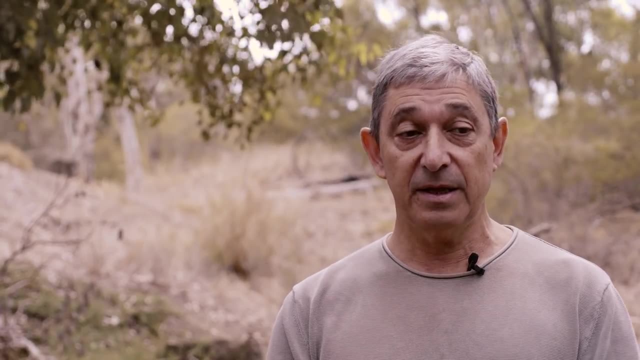 Malleefowl are socially very monogamous. They tend to have, you know, long-standing pair bonds. That in itself is quite unusual amongst birds, but not totally unusual. What makes it really quite unusual is that the male and female are forced to spend a lot of their time during the breeding season apart. 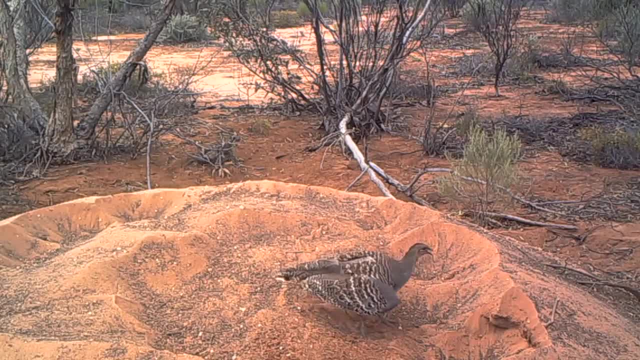 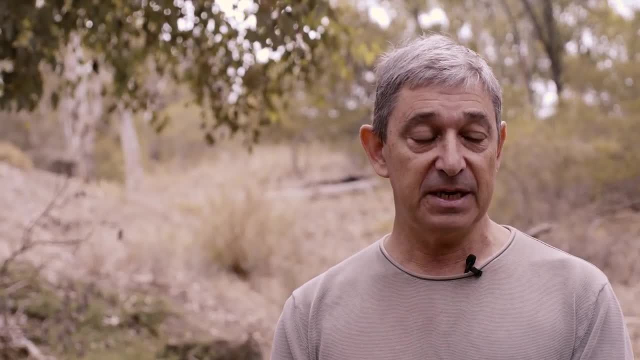 Usually that wouldn't happen in the animal world because particularly the males will try and guard their female and make sure nobody else you know gets in there and fathers eggs. But Malleefowl have no choice. They're locked into this breeding system. 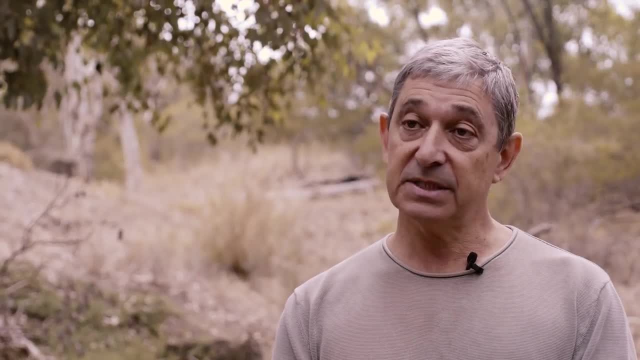 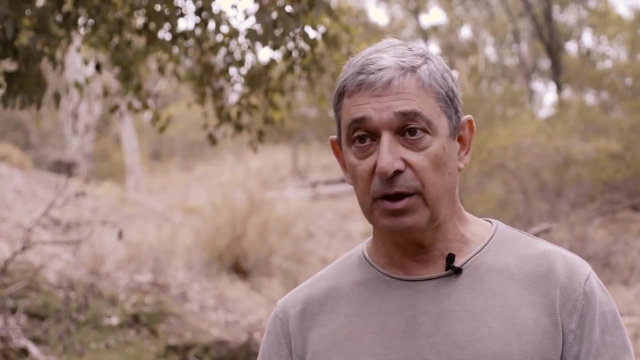 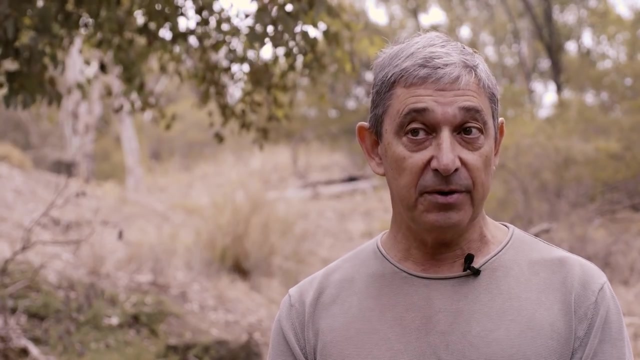 and the only way it can work now is if the male stays with the mound and basically maintains the mound, maintains the temperature in the mound, so opening and closing every day. The female has an equally big challenge and that is to find the food to make her eggs. 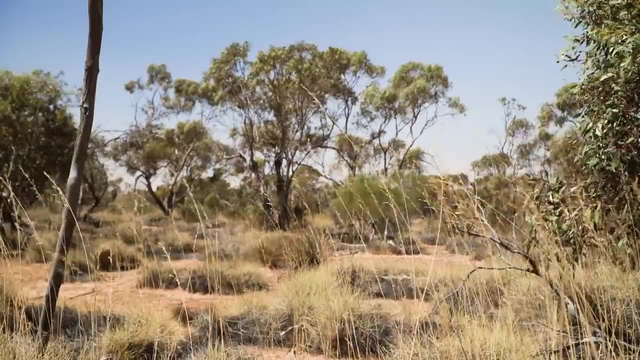 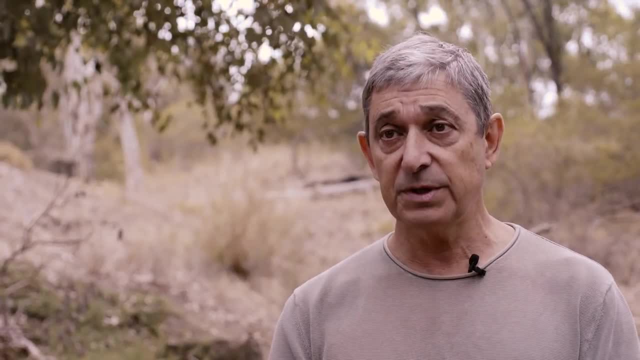 because in the Mallee it's very dry- There's no surface water, typically- And yet the eggs are huge and of course they're full of water and they're also full of protein and energy. So the female has to try and find the food to make the eggs. 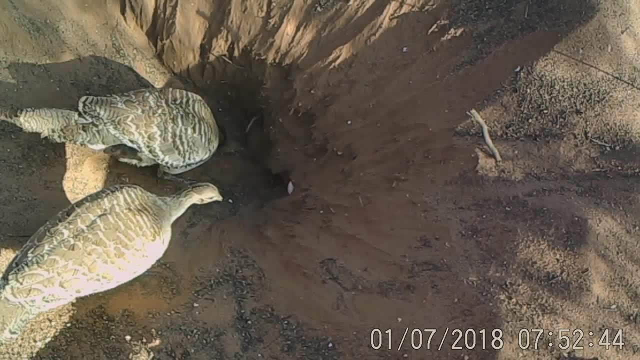 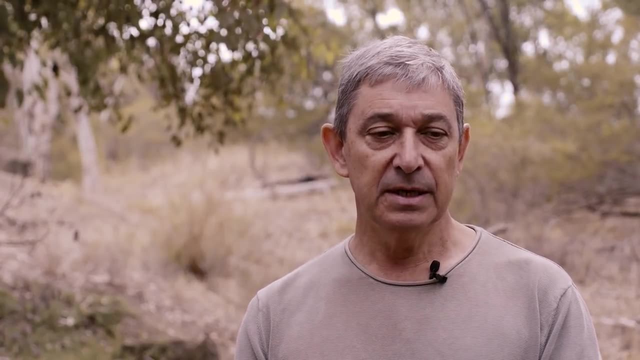 The Malleefowl aren't much bigger than, say, an Isar Brown, a little bit larger with a longer neck, But we're still only talking about a kilo and a half to two kilos, And they produce an egg, that is you know. 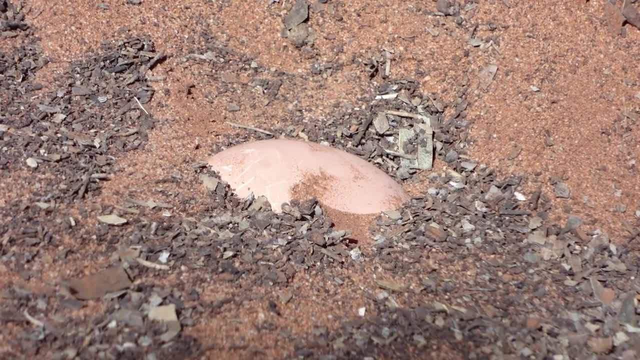 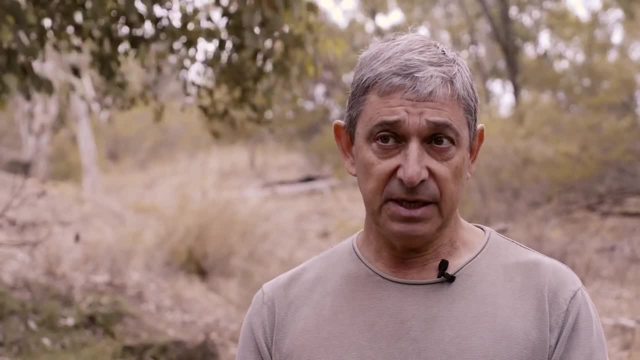 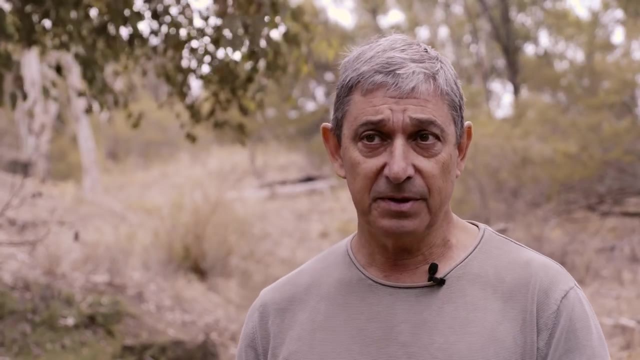 maybe three times the size of a domestic chicken, So a huge egg Around about seven to ten percent of the female body weight, And she does this every three days or so. So it's analogous to childbirth, which is, I think, also roughly in that ballpark. 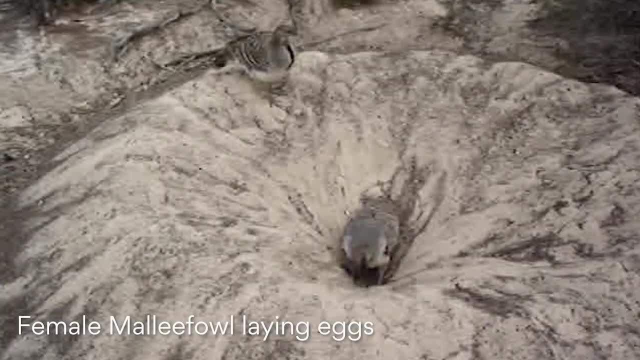 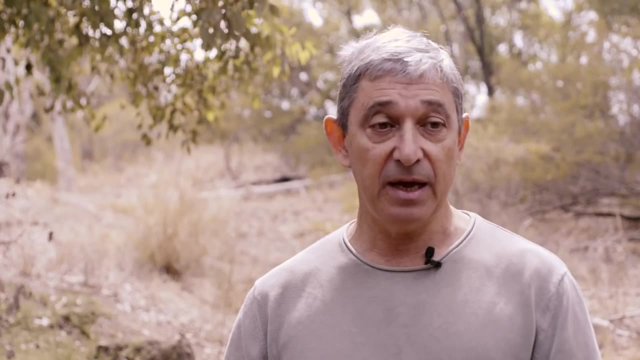 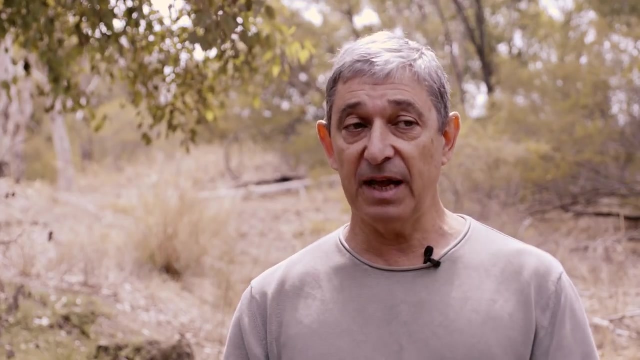 Only Malleefowl are producing these eggs every three days, So it's a huge investment. Within a season she may lay two or three times her own body weight in a period of a few months- Unbelievable effort. And this is done largely over spring and summer in the Mallee. 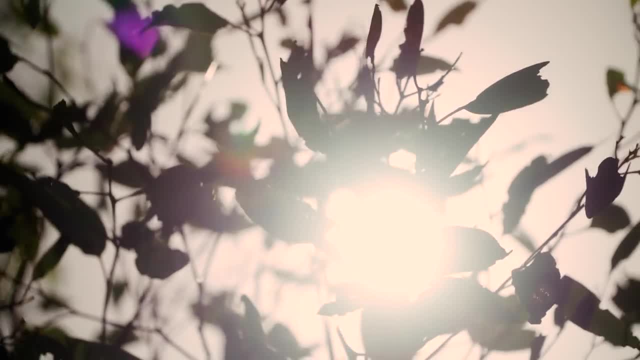 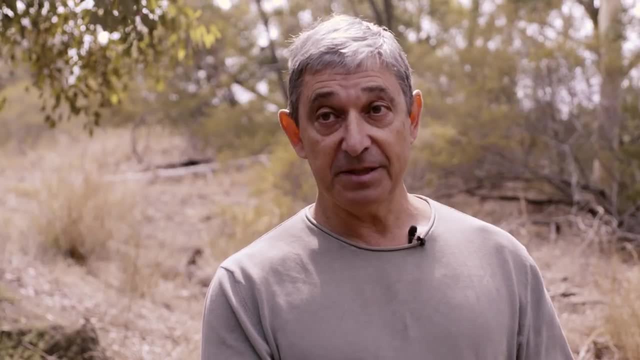 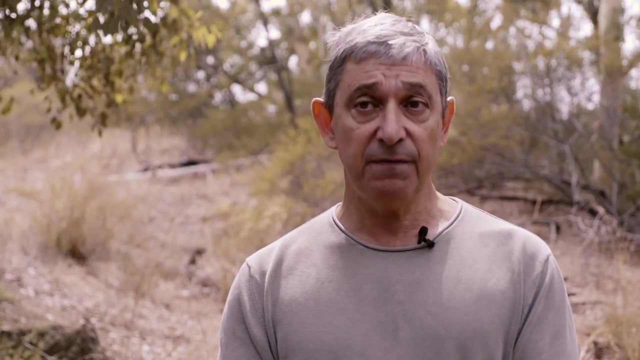 which are dry and fierce times. So it is in itself quite astonishing, Malleefowl. you know, while they're looking after the eggs in the mounds, they're doing a brilliant job. Very, very high survivorship. Survivorship of the actual eggs is typically very, very high. 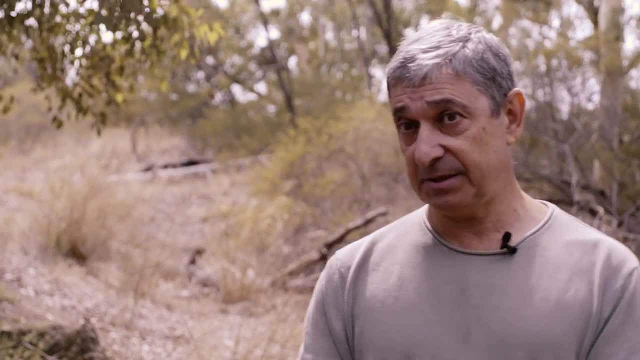 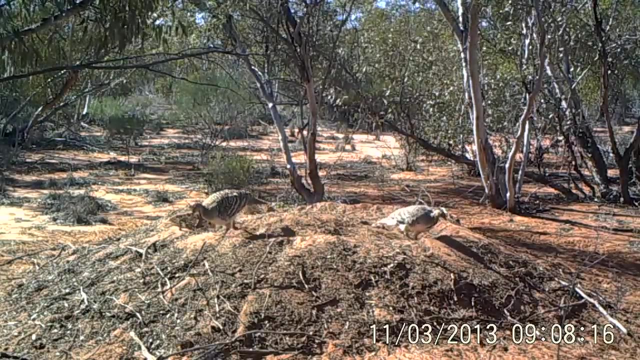 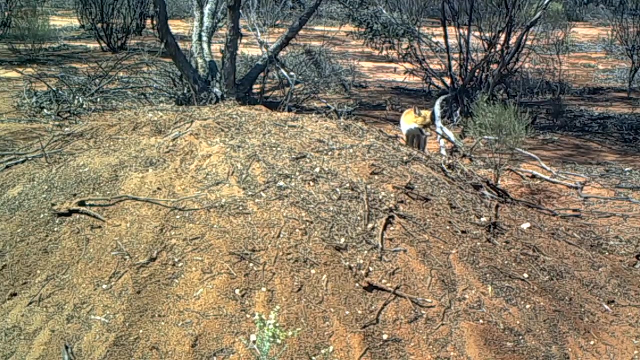 Much higher than it is for birds in nests. as a general rule, Seventy to eighty percent is quite normal hatching success from Malleefowl mounds, And although you would think that things like foxes would quickly get into mounds and gobble up all the eggs, 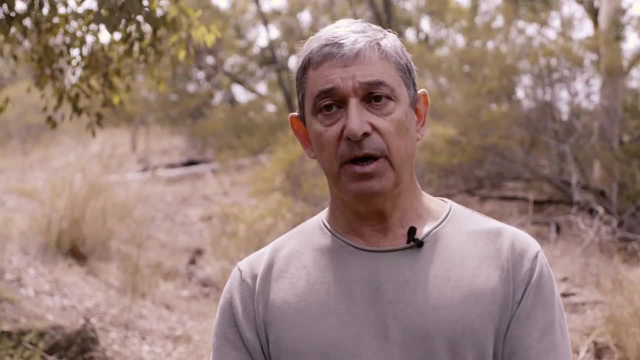 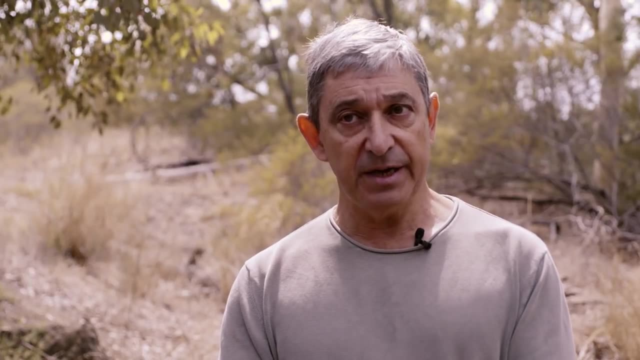 and they do occasionally. the predation on eggs is actually fairly minor. In some years it goes through the roof, and when I say through the roof, they might take a third of the eggs that are laid, But in most years it would be under five percent of the eggs that are laid. 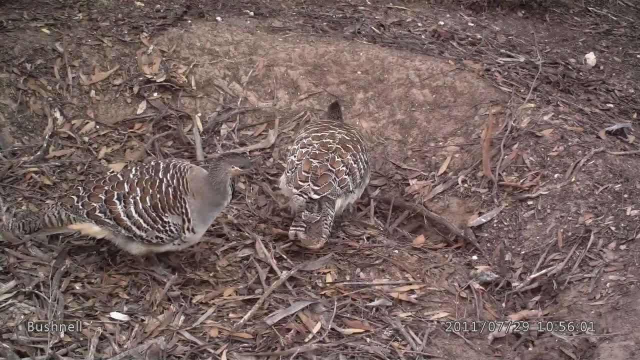 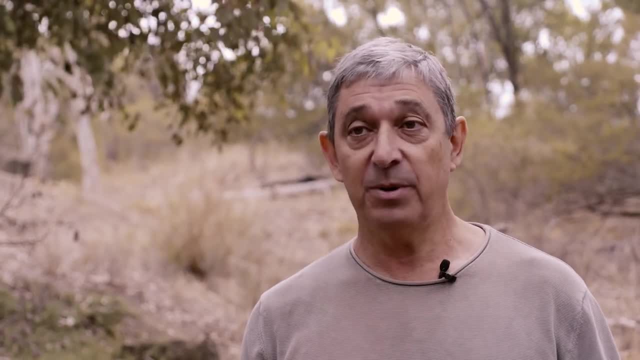 There are many, many extraordinary things about Malleefowl. Another one of the astonishing things about Malleefowl is they have once the chicks come out of the eggs, there's no parental care. When the chicks come out, they actually dig themselves out. they hatch out. It can be up to a year. It can be up to a meter under the surface. They have to find their own way out. They're buried in sand. They have the advantage, though, that the male remember. 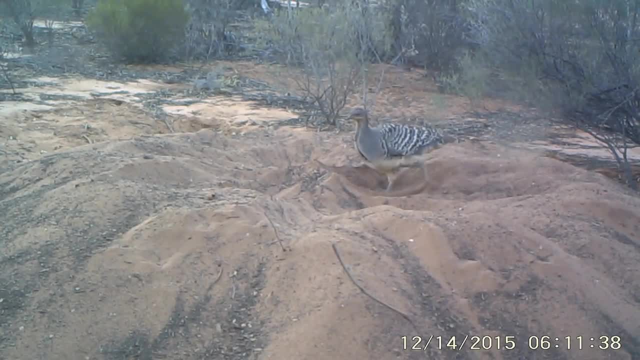 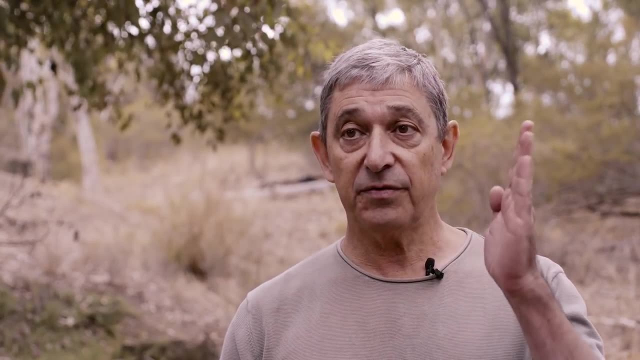 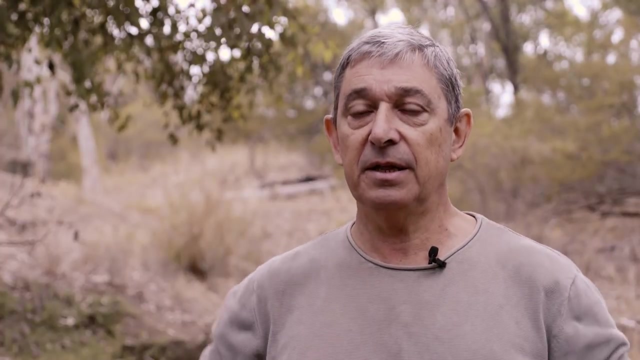 is moving the sand probably every second day, checking the temperature, closing it up again. so it's all loose sand And the chick has to kind of dig its way out or, if you like, just float its way out, moving and wriggling so the sand keeps going underneath it. 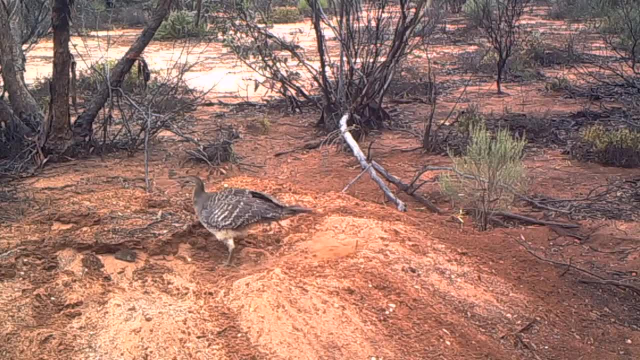 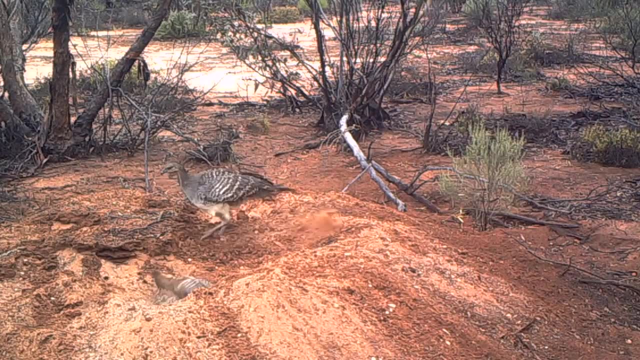 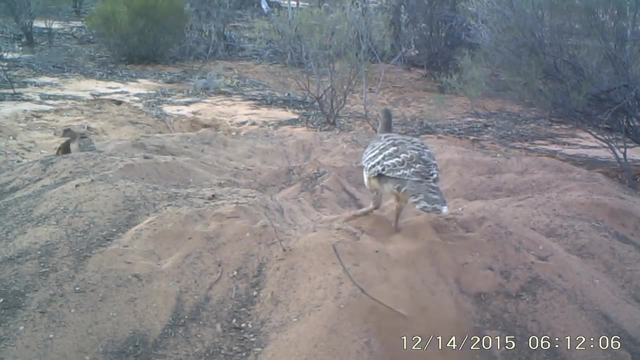 finds its way out quite comically, sometimes rolls down the side because by this stage it hasn't walked yet. and it can't often walk, can't stand up, But the damn thing can run and can run really fast and can even fly on the first day. 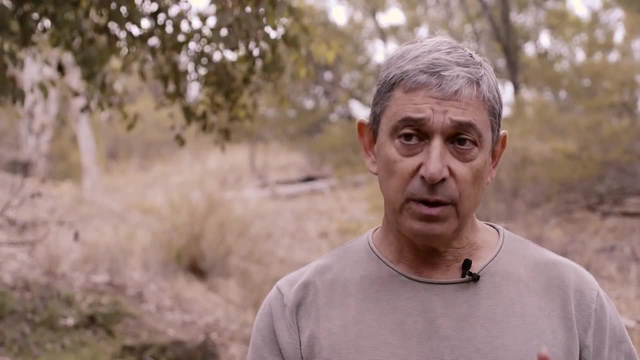 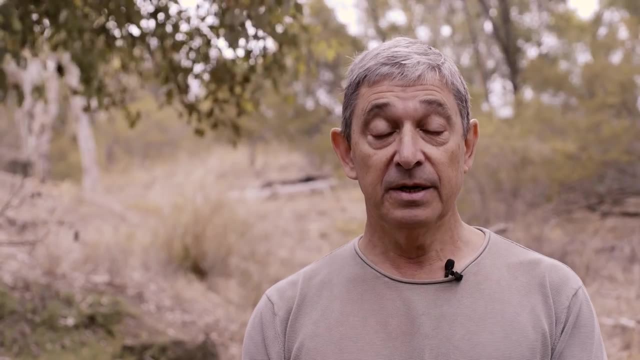 usually quite low to the ground. So these are really well-formed chicks that come out no parental care and the Mallee is a pretty inhospitable place in summer. So these chicks- you'd think the chances of them surviving are very, very low. 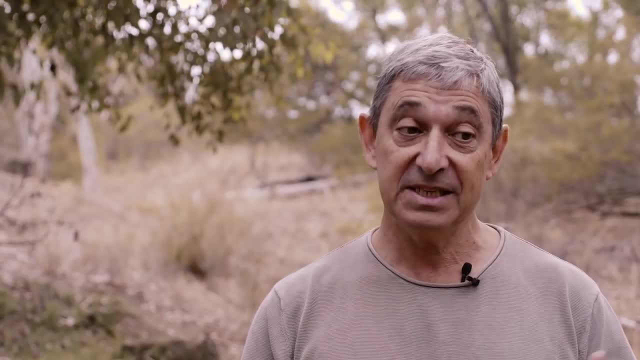 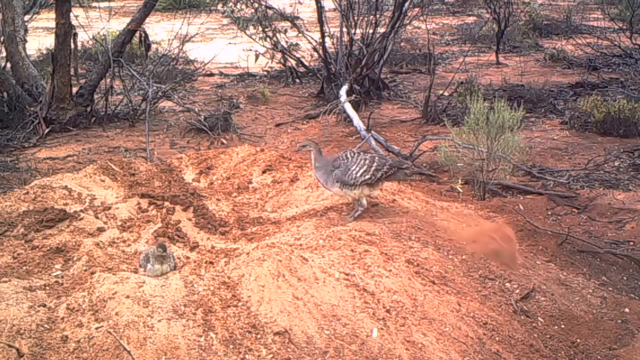 And in fact the survivorship is very, very low. but it's a system that seems to work very well. Things sort of go wrong, or at least they get hard for a baby Malleefowl. when it leaves the mound It still has some yolk in the belly. 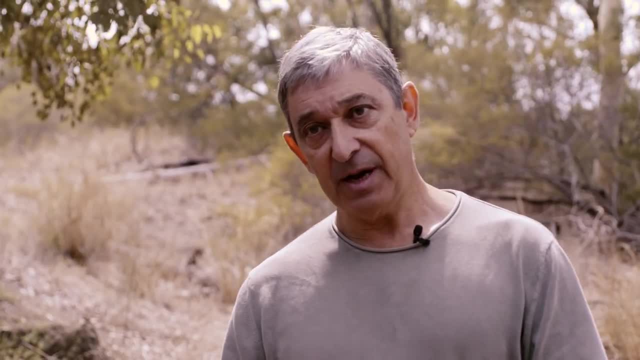 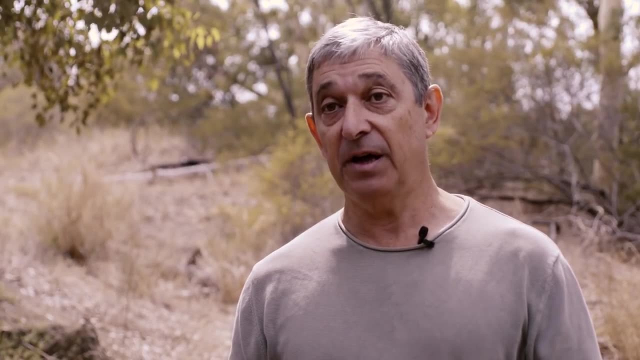 so in a sense it's got, you know, like I say, it's got a little cut lunch for a couple of days and it's got two or three days to find food, And if it doesn't find sufficient food in that two to three days. it's going to go hungry, And that means that it'll eventually starve- and quite a few chicks starve- or it'll be picked off by predators because it's out looking for food, Whereas a chick that has found food will rest most of the day. 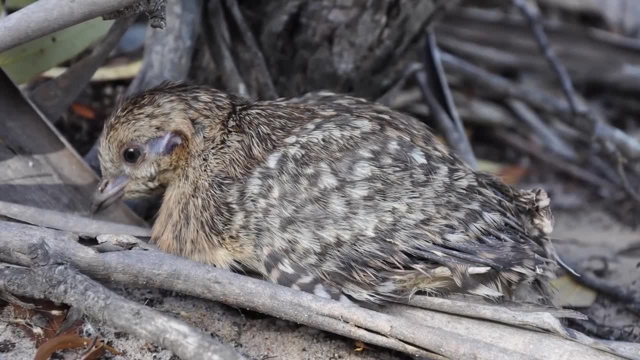 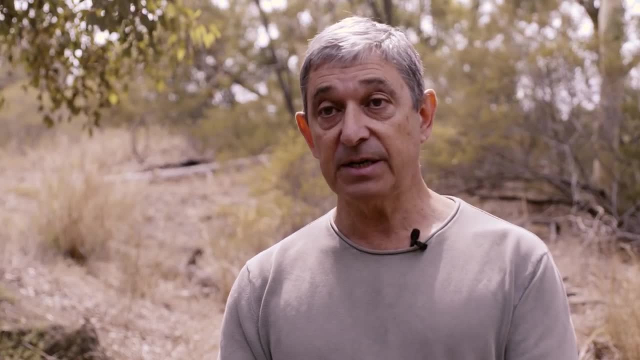 and they just disappear. Malleefowl have the most fantastic camouflage. They will completely disappear in the leaf litter and just come out for an hour a day to eat and then go back and grow. Those first few months are not just about survival. 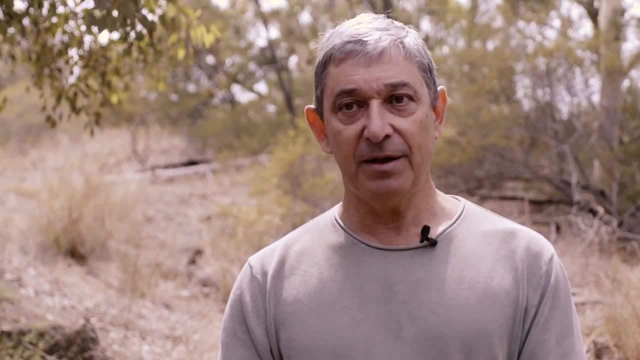 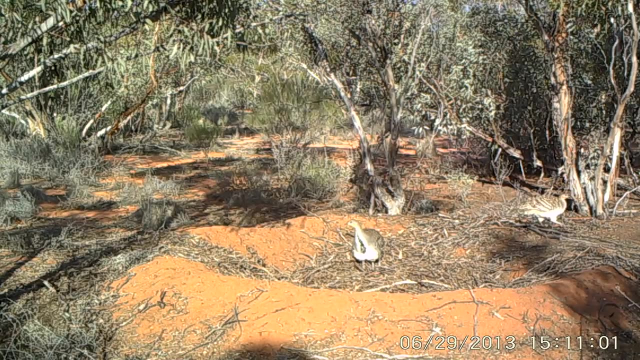 They're also about learning. There's a reason why the birds that get through are so tough, and that is because they've gone through a really tough initiation. The average life expectancy of a Malleefowl is probably about two to three weeks. 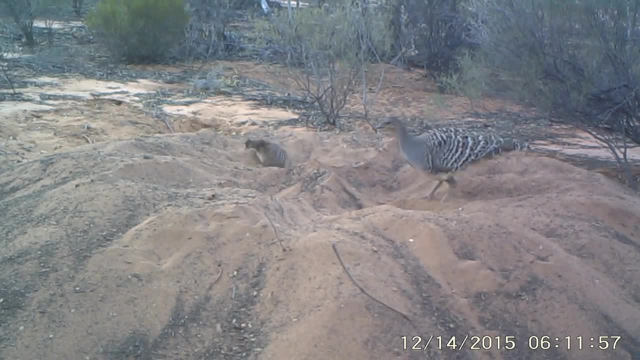 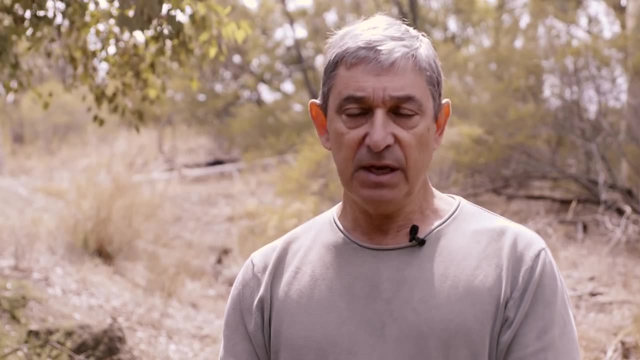 Most of the chicks die. Most of the chicks die because it's a terribly harsh environment and full of predators. Everything's out to get them for quite a while. If they do survive the first six months, then once they get to adult size, 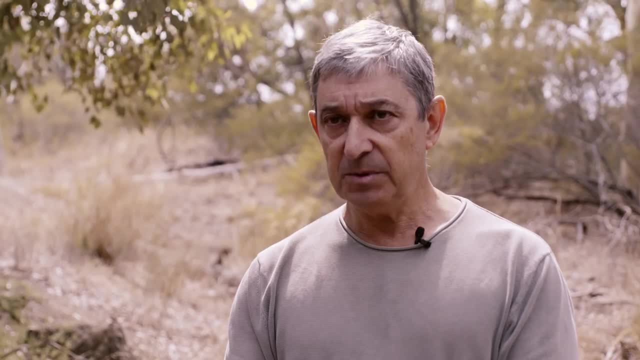 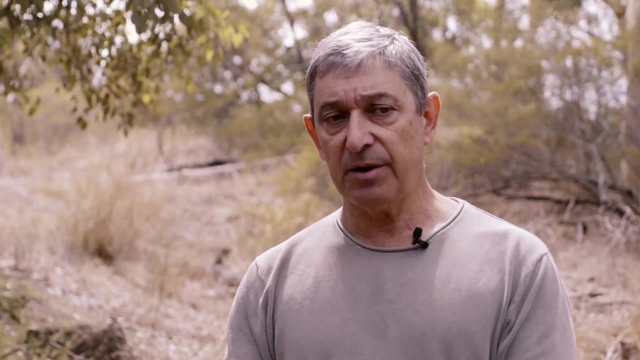 you know of a year or so. they seem to be pretty good for quite a few years. They seem to live in the wild. our best estimate is, you know, 15 to 20 years, And we're just talking here of breeding birds. 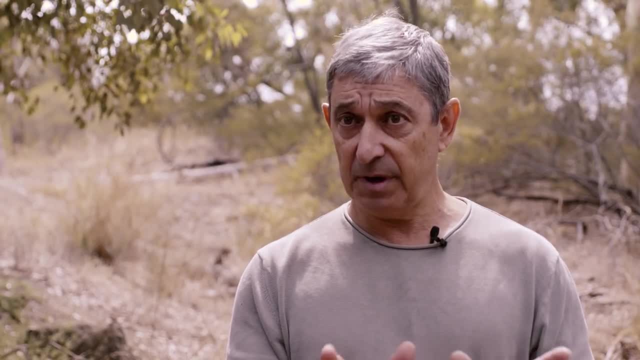 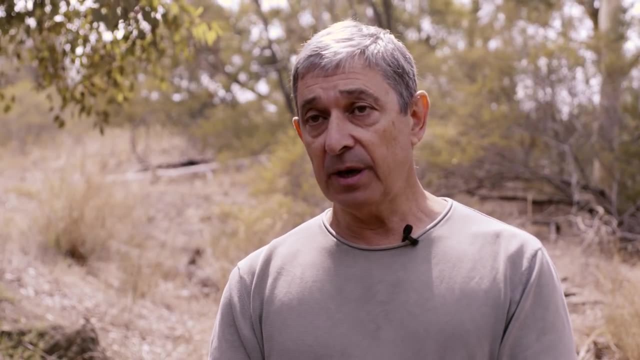 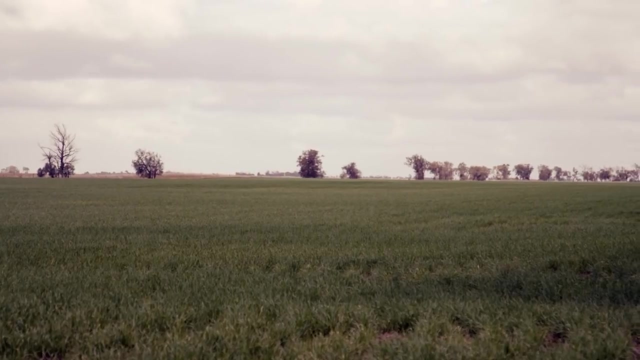 So 15 to 20 years, you know, average life for a breeding bird is pretty good. Populations are slipping And we know that. we've measured it. Populations are slipping even in habitat that hasn't been cleared or altered. 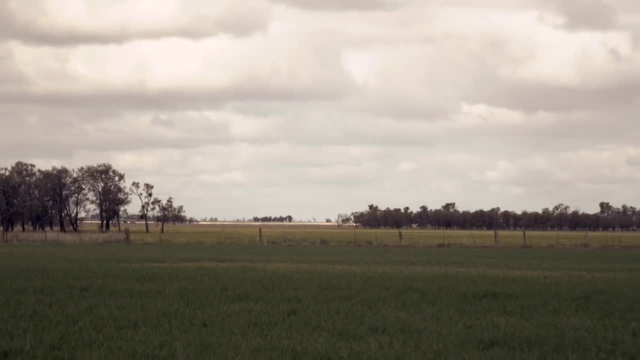 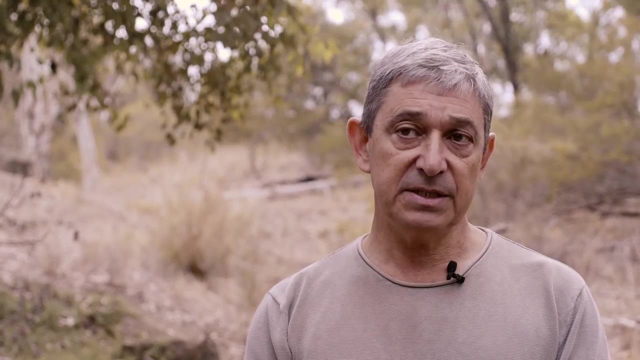 In the wheat belts of Australia that once contained some of the best Malleefowl habitat. most of that habitat is all gone. The biggest threats now are the introduced the invasive species that we brought in. Foxes in particular are a great concern. 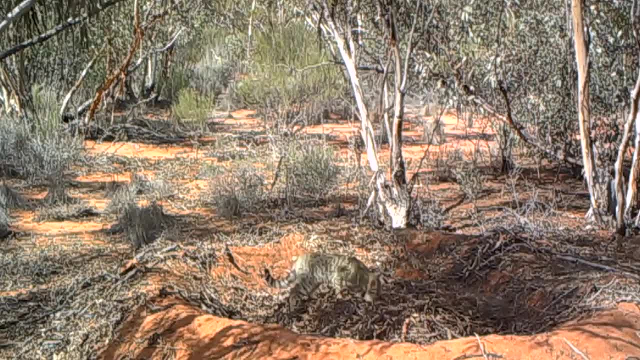 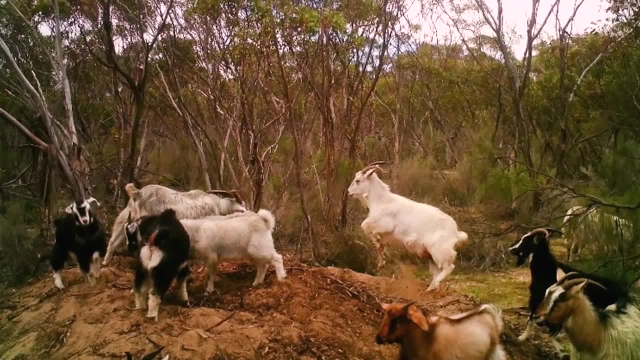 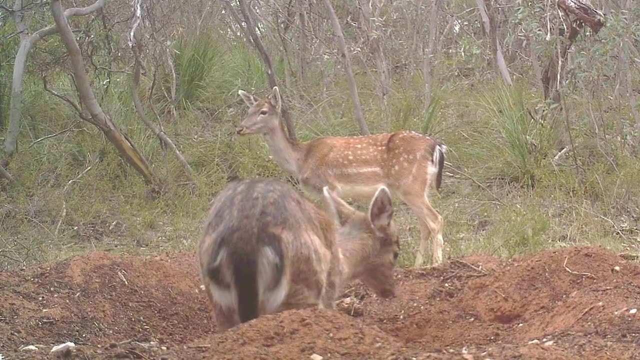 but cats are also a great concern. And then a lot of the introduced herbivores: Goats are a major problem in a lot of areas, But also sheep and rabbits, and we have pigs encroaching on other areas and deer encroaching on other areas. 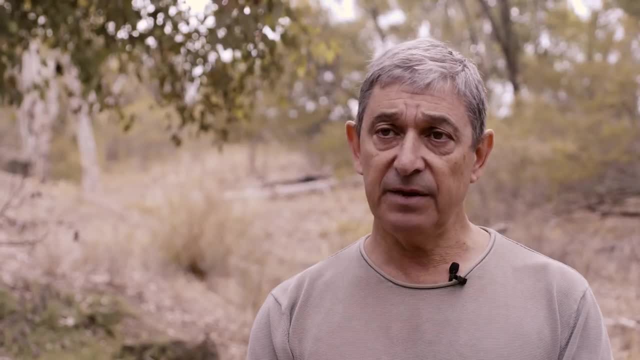 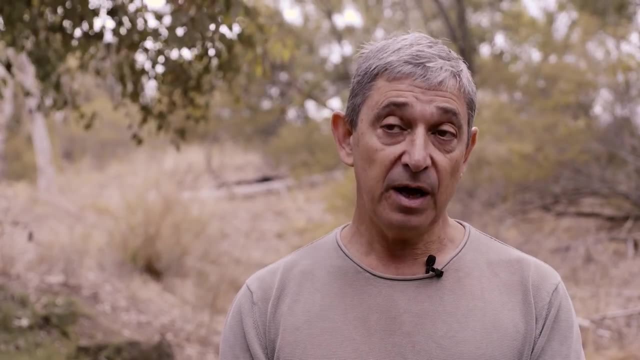 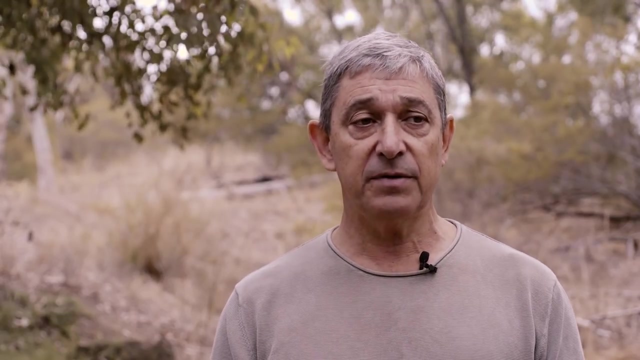 The herbivores can make a very strong negative impact because they're the same food that Malleefowl eat. There's actually quite a long list of threats. Fire is a big one, While fire has always been part of the Australian landscape and is certainly part of the ecology of the Mallee. 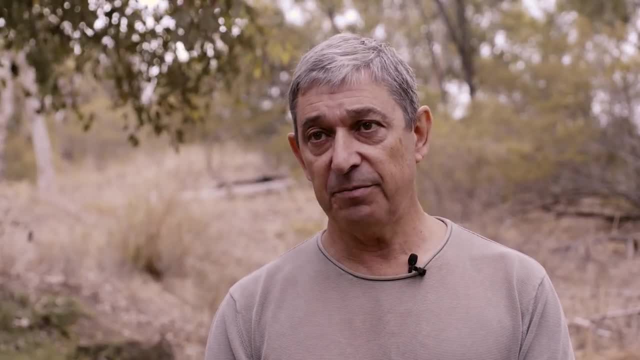 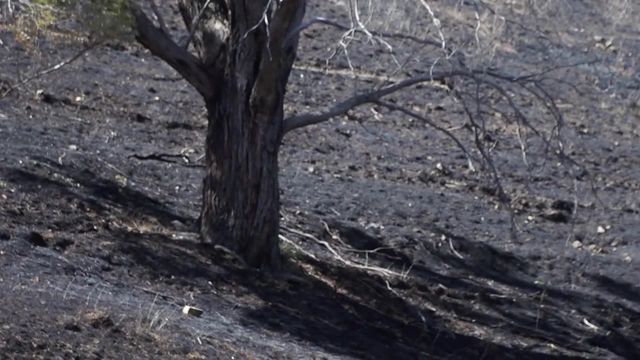 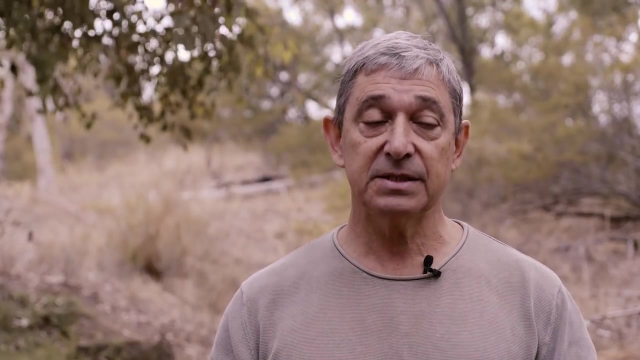 huge fires will take out a lot of Malleefowl country and a lot of Malleefowl. very, very suddenly- And that becomes important because the continuity of the habitat has all been broken up- We now have these blocks of varying sizes. 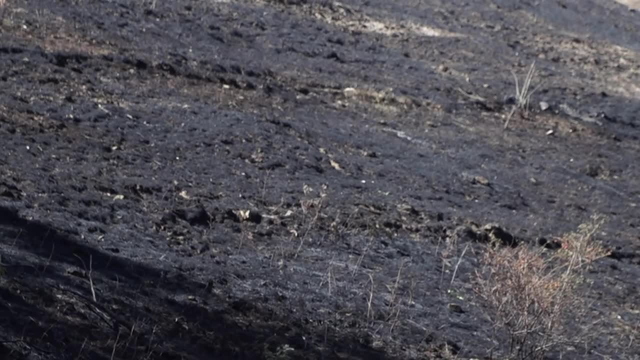 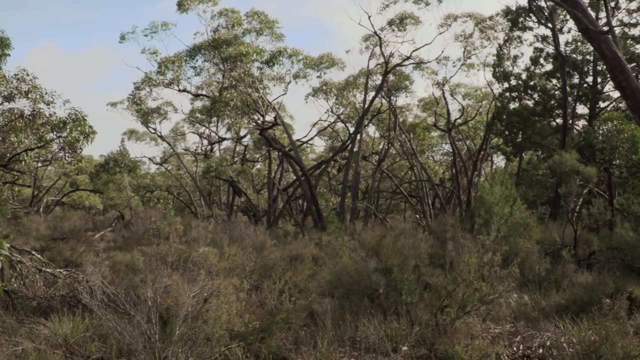 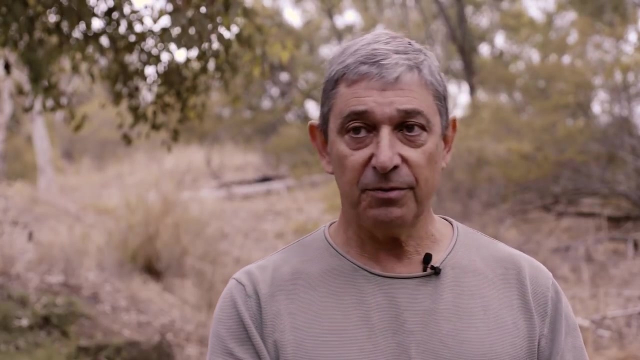 but many of them can be taken out by one fire. The biggest concern for the future is climate change, because that changes everything, Even if the same amount of rain comes in the future, if it's distributed in the summer rather than the winter, when Malleefowl need it to make their mounds. 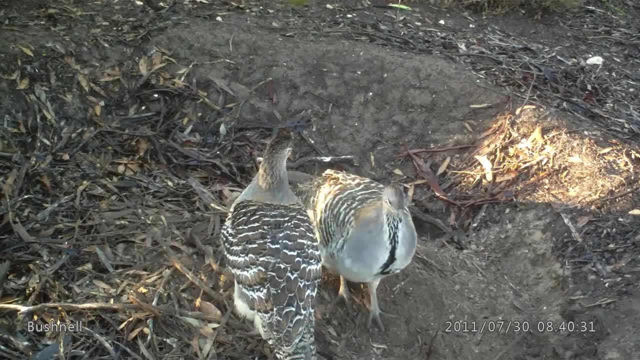 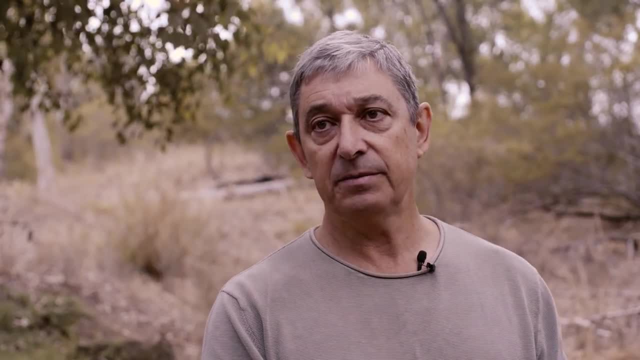 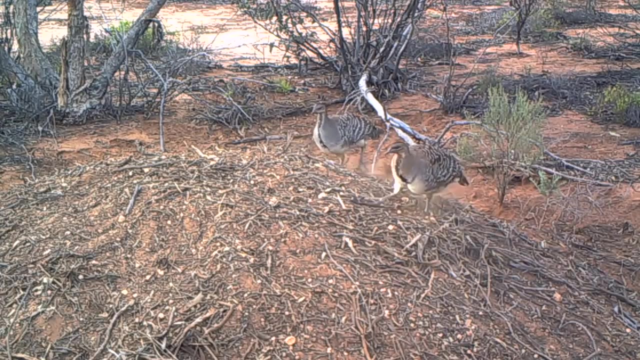 it'll have a big impact on breeding. So everything that the Malleefowl does is tuned to the environment that it has been living in for many thousands, hundreds of thousands of years. Any changes could have big impacts, not only on Malleefowl, of course, but on all of us. 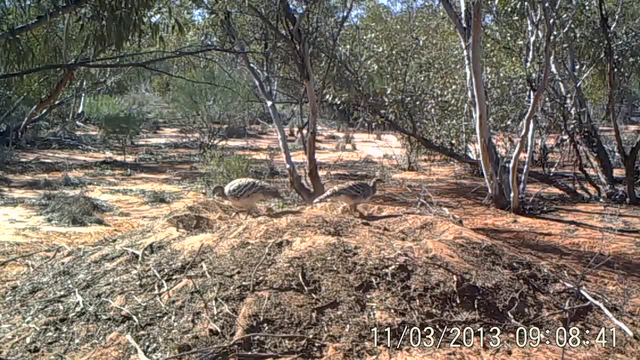 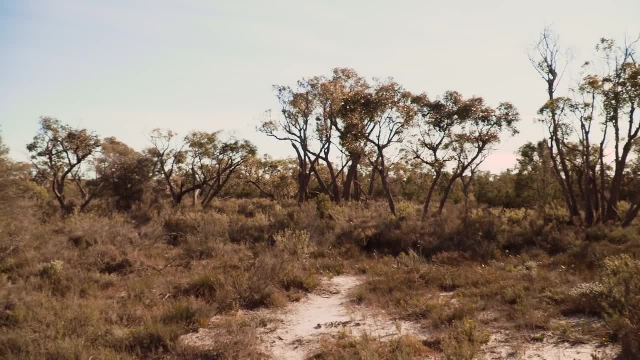 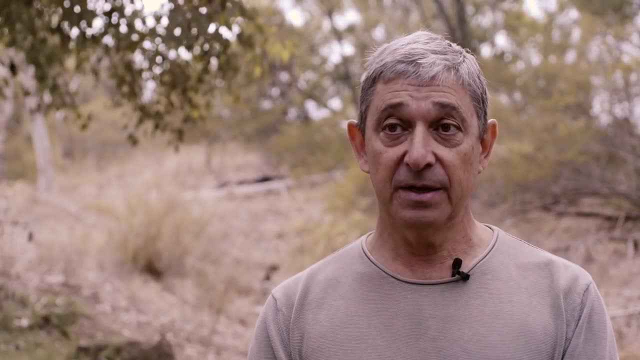 Malleefowl need rain at much the same time as the weed farmers do. We are all part of an intricate web. I think it was when I started working in central Australia that I really started to understand how incredibly tough these birds are. You sometimes get the impression.